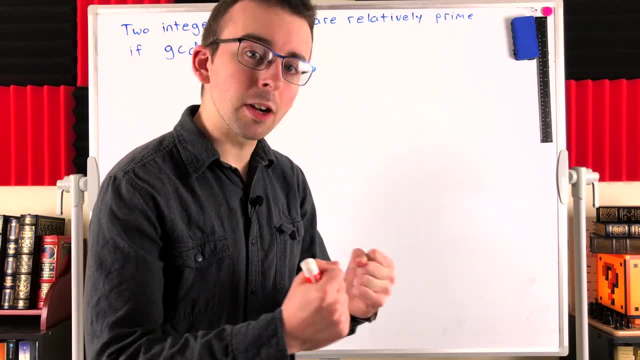 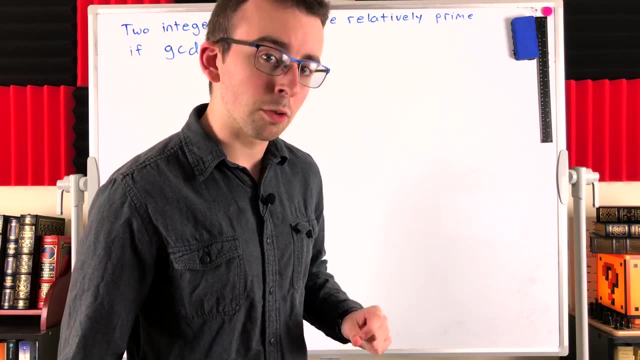 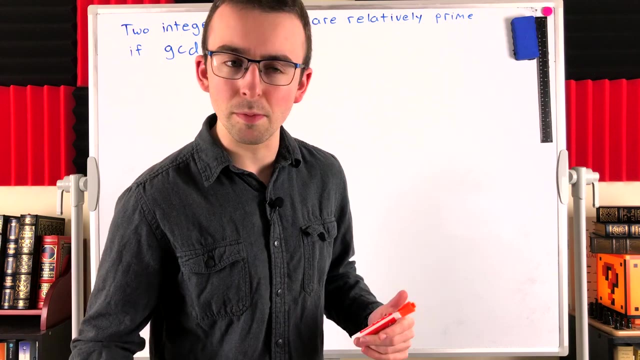 divisor of every integer. so every pair of integers do have a divisor of 1 in common. If 1 is the only positive divisor they have in common, that's what makes them relatively prime. So start to think on our question: is 1 relatively prime to itself? Another way we could state the 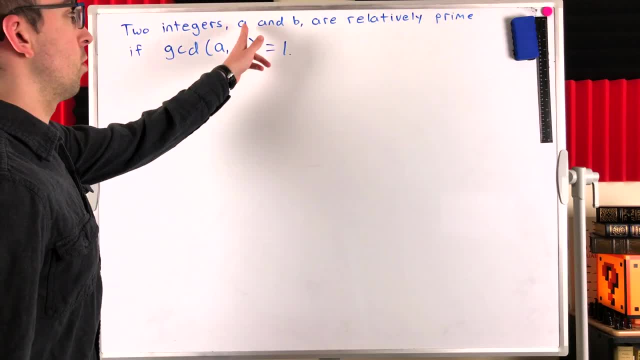 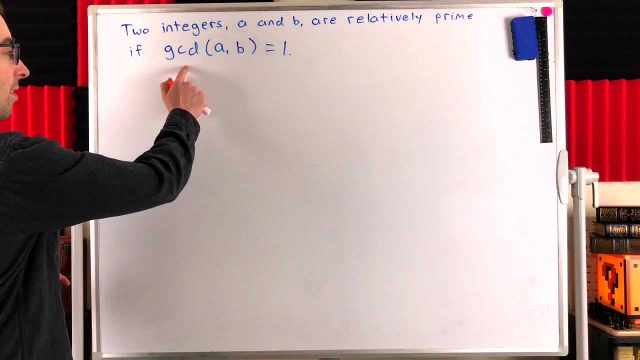 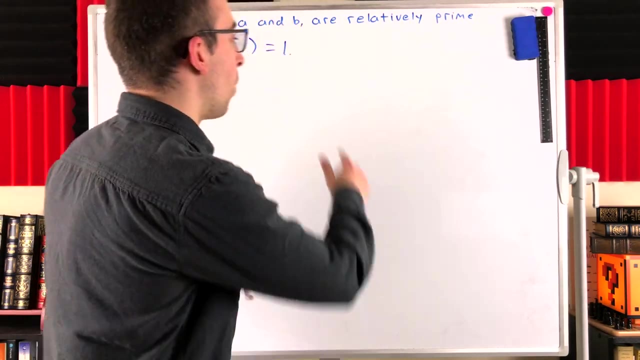 definition of relatively prime is like this: Two integers, a and b, are relatively prime or mutually prime or co-prime, if their greatest common divisor, so the GCD of a and b, is equal to 1.. Certainly, if 1 is the only positive divisor of two numbers, then 1 is their greatest. 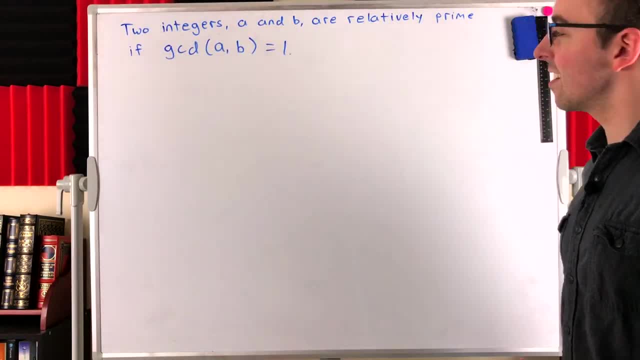 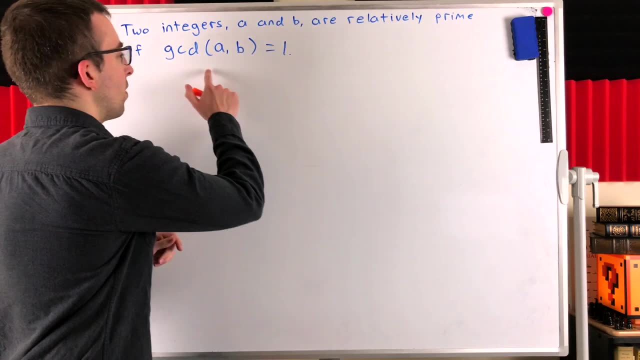 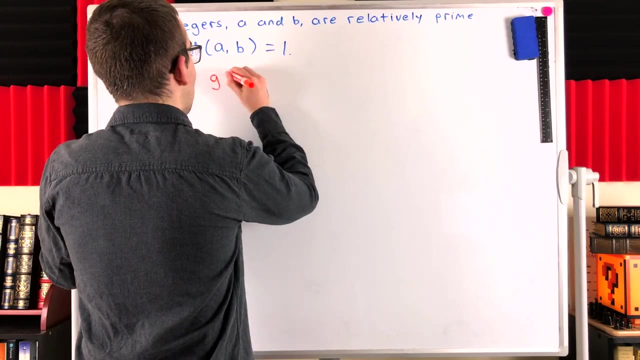 common divisor. So that's just another way that we can state the definition of relatively prime. So is is this true about one and one is the greatest common divisor of one and one equal to one. Well, we can actually push that a step further instead of just answering that question. 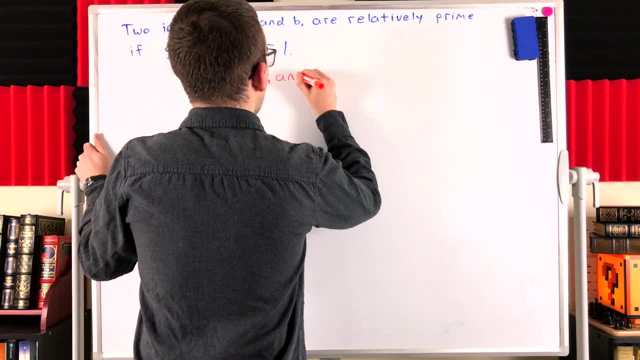 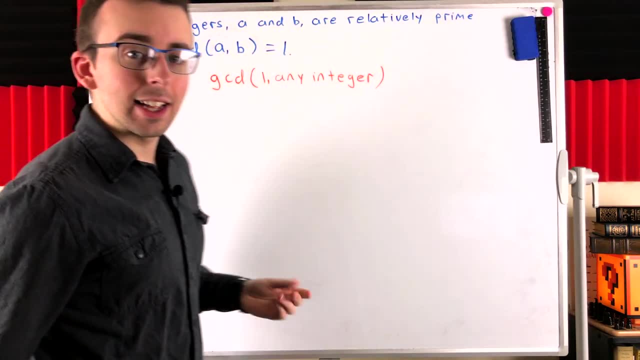 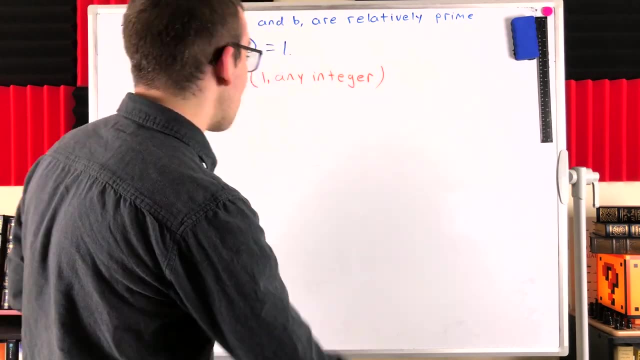 what is the greatest common divisor of one and literally any integer? Well, one is a divisor of any integer, one divides every single integer and one is the only positive divisor of itself. So, necessarily, the greatest common divisor between one in any integer has to be one. 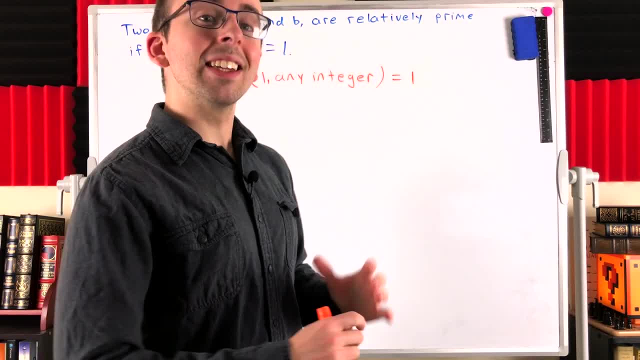 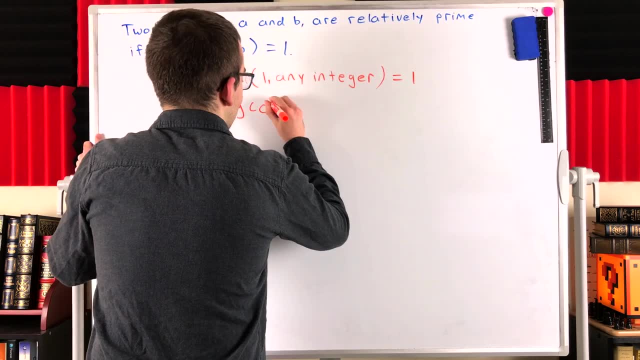 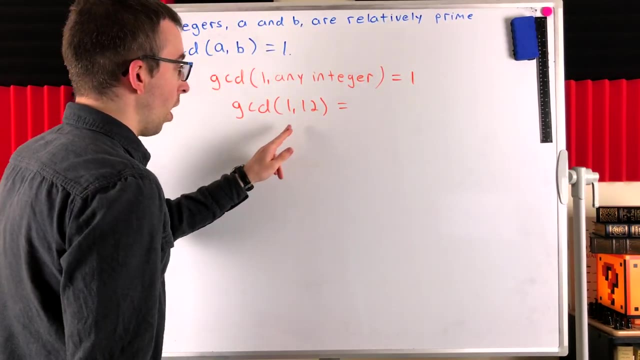 So, in fact, one, by definition, is relatively prime to every integer which includes itself. So, just for an example, what's the greatest common divisor of one and 12?? Well, one is a divisor of both one and 12.. And one is the greatest divisor of one. So it. 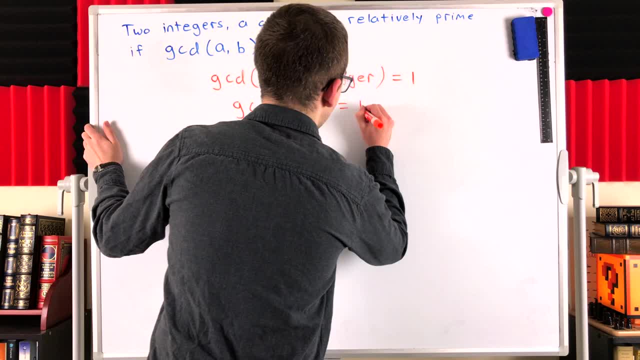 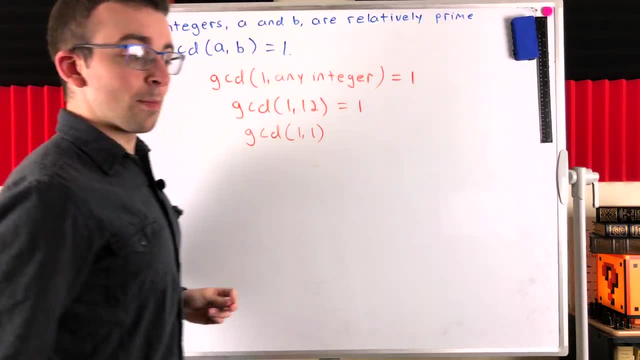 is the greatest common divisor of one and 12.. And so one and 12 are relatively prime. And then, directly addressing our question: what's the GCD of one and one? Well, clearly, it's one, that's the only positive number that divides one. So it's: 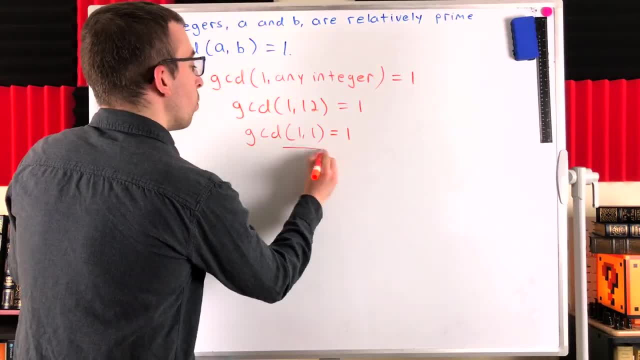 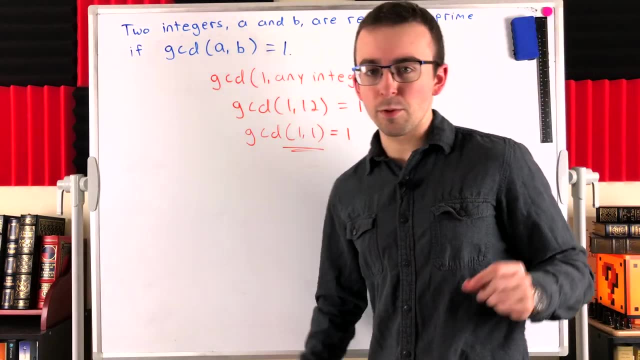 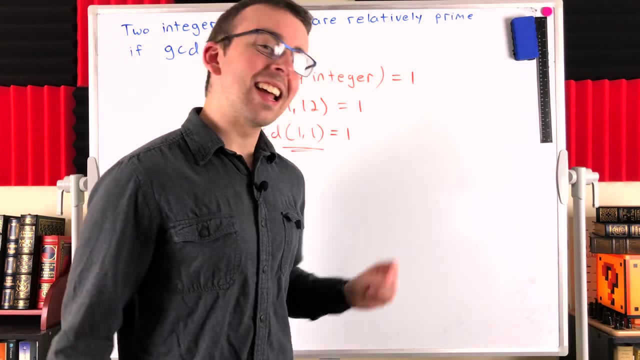 the greatest common divisor of one and one, And so one and one are, by definition, relatively prime. That's the answer to the question. One is relatively prime to every integer. There's actually another integer that has the same property. What integer do you think it is? Of course it's negative.